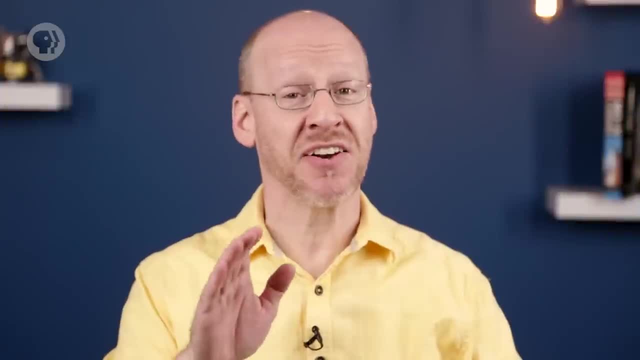 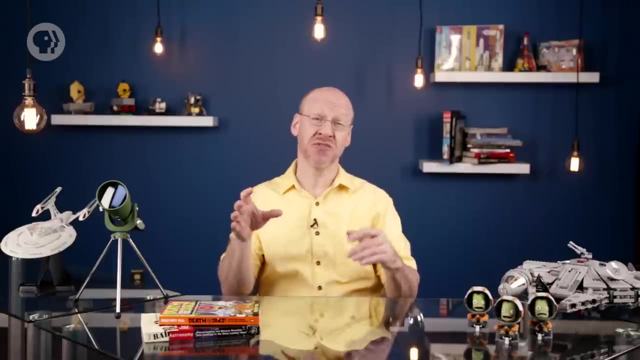 as well as the atmosphere being deeper than Jupiter's too. That's not to say, Saturn doesn't have storms. Oval hurricanes pop up every now and again, and in 2010, a huge storm erupted in Saturn's northern hemisphere. It was discovered by an amateur astronomer, and Cassini spacecraft pictures showed it. 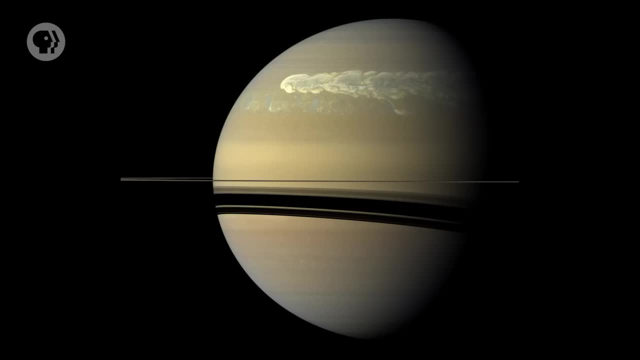 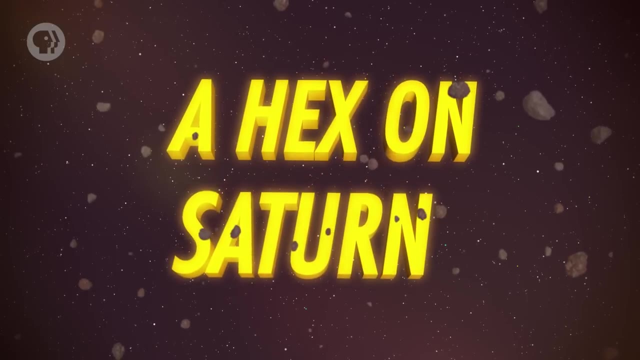 getting so big it literally wrapped around the planet, reaching a length of over 300,000 kilometers. Traces of it persisted for years. One of the most striking features on Saturn is a huge hexagonal vortex at its north pole. Vortices like this are common on planets. Earth and Venus have them too. That well-defined. 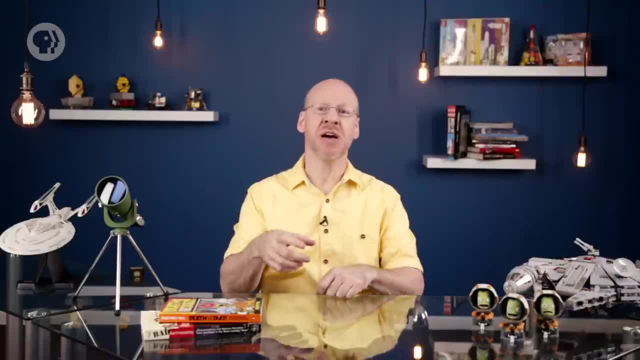 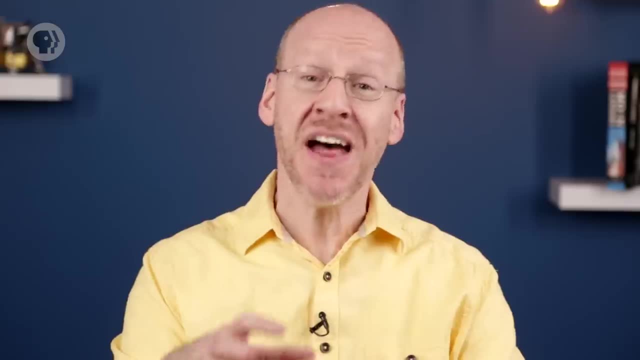 six-sided shape is pretty freaky, but it's actually a natural outcome of a spinning fluid – the air circulating in Saturn's atmosphere – which itself is in a spinning system, in this case the planet itself. It's not that different than Earth's jet stream, but it's a lot bigger: about 20,000. kilometers across, wider than Earth, And right at its center, over Saturn's north pole, is a ridiculously beautiful storm system, about 2,000 kilometers across. Wind speeds there have been clocked at 500 kilometers per hour. Saturn as a planet is, of course, an amazing place, but come on, When you think Saturn. 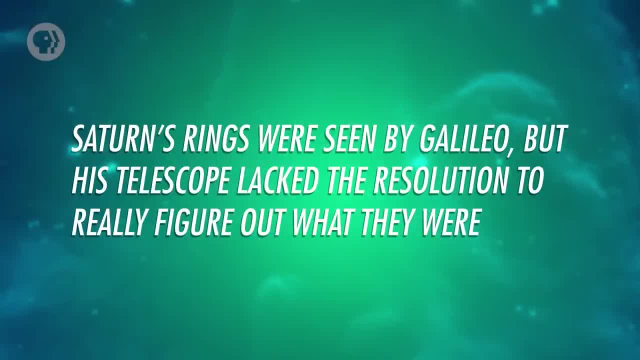 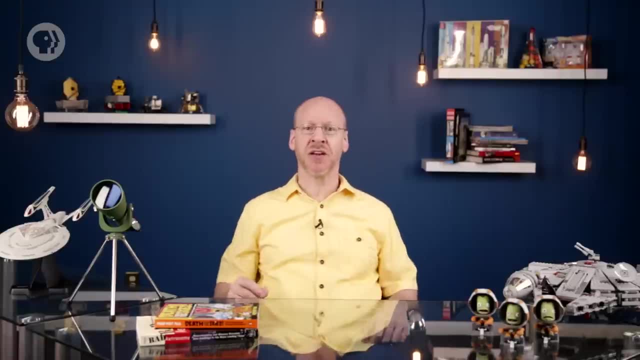 you think rings As well you should. Saturn's rings were seen by Galileo, but his telescope lacked the resolution to really figure out what they were. He thought Saturn might be three objects in close proximity. Some decades later, the Dutch scientist Christian Huygens correctly interpreted their appearance. as a ring surrounding the planet. They're not solid. If they were, they'd get torn apart, since the inner edge would orbit the planet way faster than the outer edge. They're actually made of countless small chunks of very nearly pure water: ice- Each particle. orbits the planet independently, So I guess Saturn wins in the which planet has the most moons category. What really gets me about Saturn's rings is their scale. They're 250,000 kilometers across. If you put Saturn between the Earth and Moon, the rings would cover two-thirds. 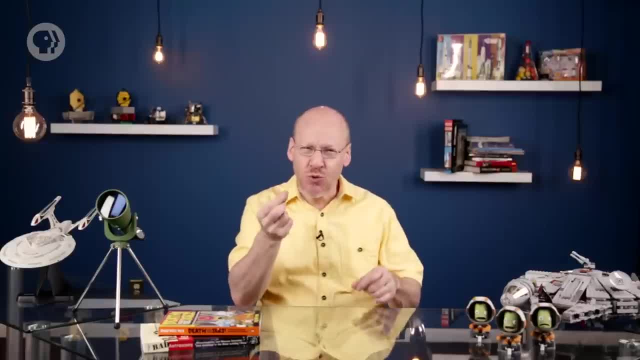 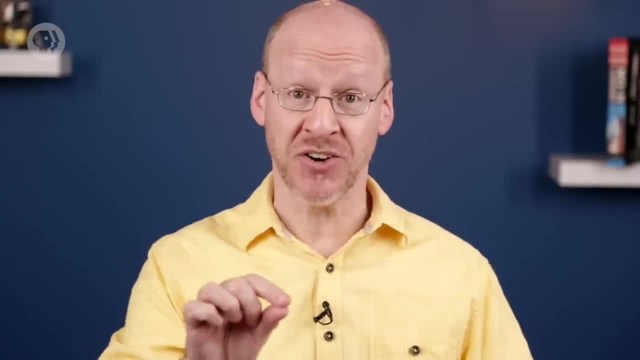 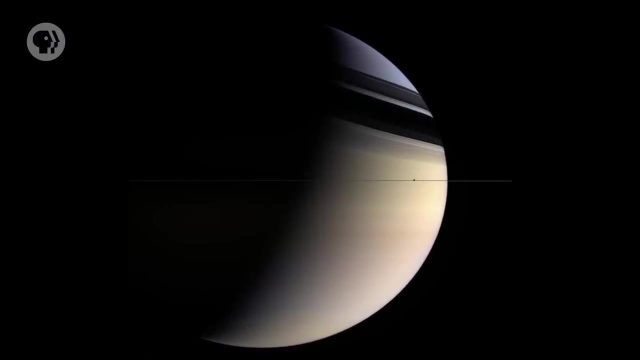 that distance And yet, despite their size, they're incredibly thin. They average about 10 meters thick. And no, I did not misspeak, I meant 10 meters. 10 meters, That's amazing. That's thinner to scale than a sheet of paper, Way thinner If you shrank Saturn down to. 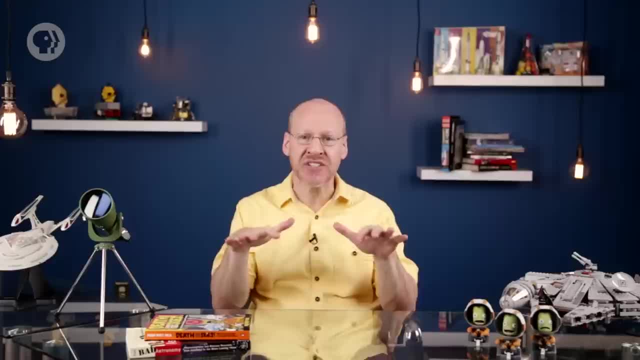 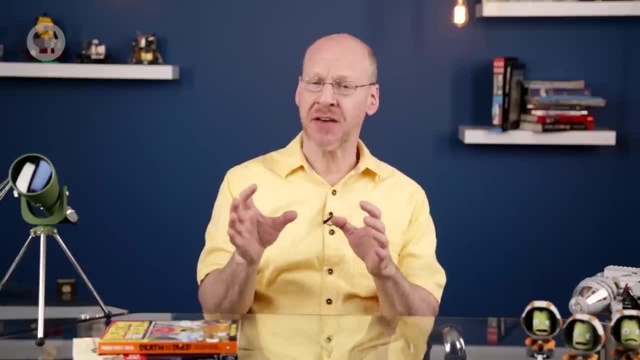 the size of a piece of paper. that paper would be 10,000 times thicker than the rings. So yeah, Saturn's rings are flat, But why? Well? that's tied to their origin. though the specifics of how they came to be aren't exactly known, One idea is that they were. 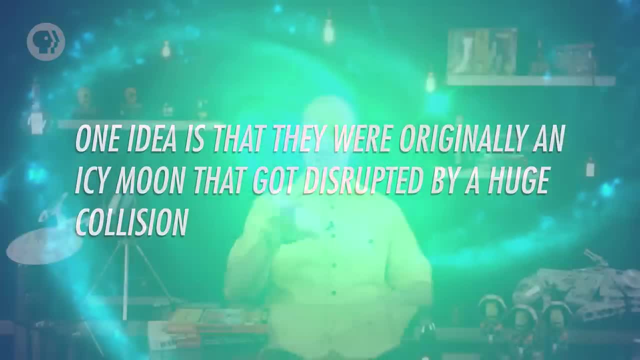 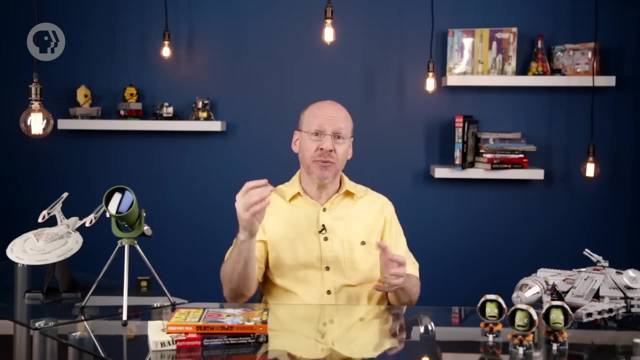 originally an icy moon that got disrupted by a huge collision. The shattered moon particles would have spread around Saturn and any of them that were on a tilted orbit would quickly collide with others and in the end that would average out all their orbits to form a flattened 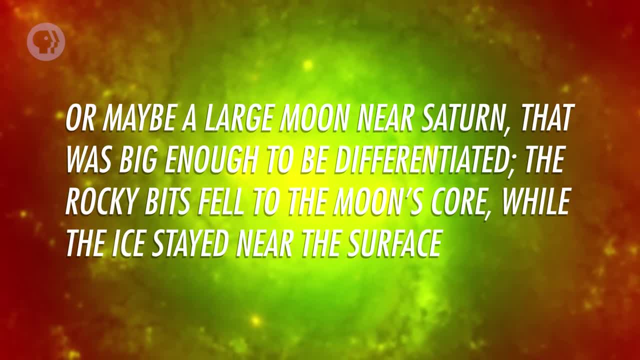 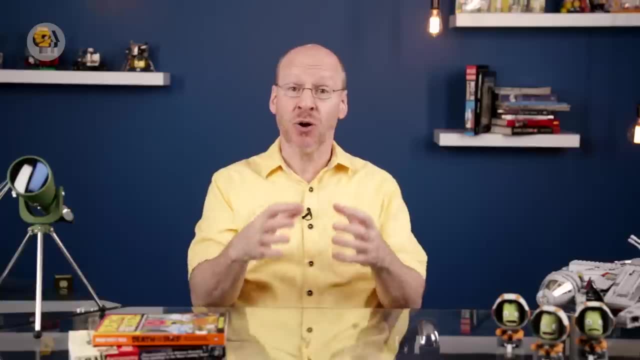 ring. Saturn has a large moon near Saturn that was big enough to be differentiated. That means the rocky bits fell to the moon's core, while the ice stayed near the surface. As it plowed through the material around the proto-Saturn, the moon's icy layer got stripped off, forming 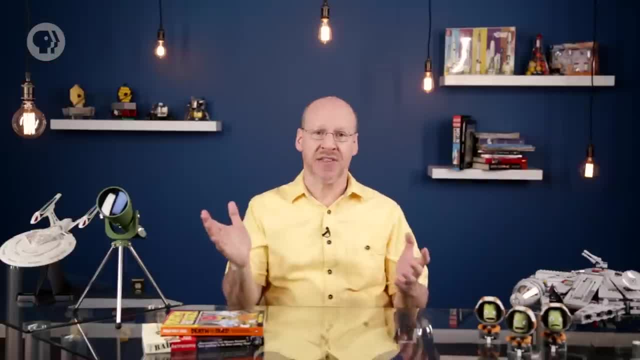 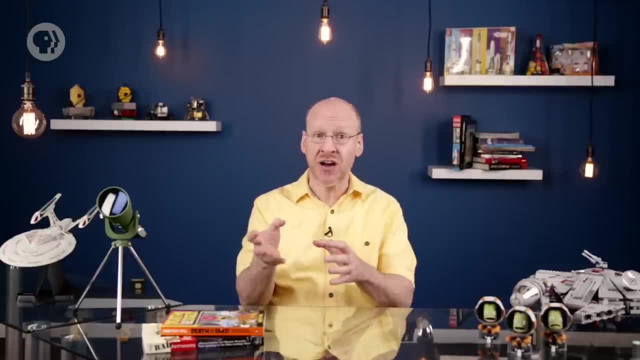 the rings And again that would form a very flat disk. However they formed, collisions would quickly flatten the ring out And remember, Saturn is oblate. so as the rings formed, they would have felt a gravitational tug from Saturn's equatorial bulge, centering them right over the planet's midline. Saturn has three main 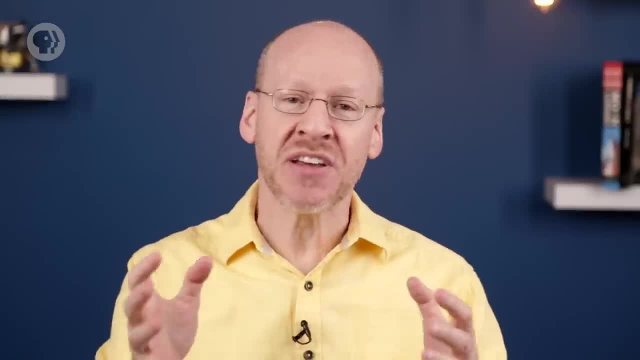 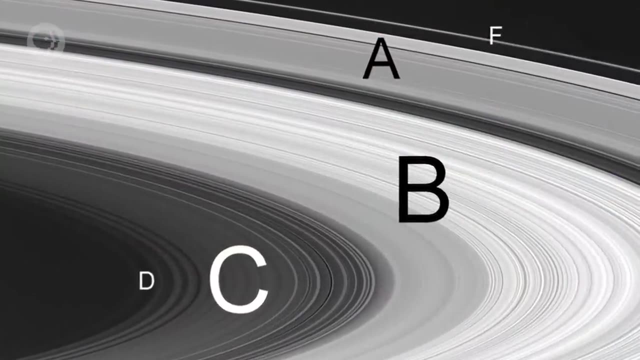 rings give or take. In classic, imaginative astronomer fashion. they're given the names A, B and C in order of their discovery. B is the broadest, roughly 26,000 kilometers wide. A is outside B, while the C ring is fainter and inside the B ring When the rings 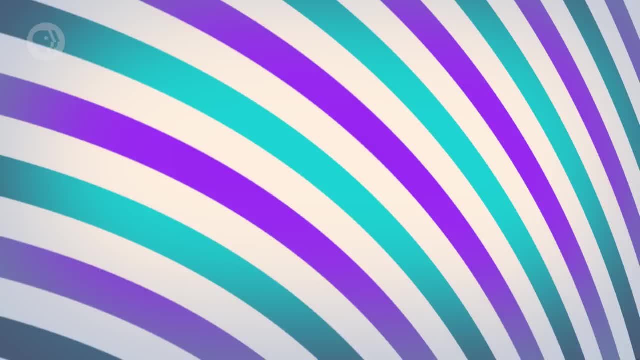 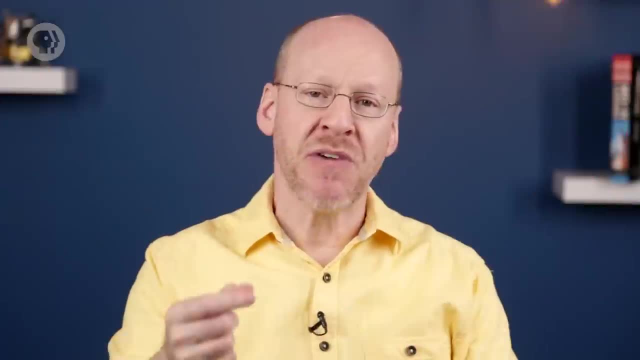 were first observed, the A and B rings were thought to be one ring, But then the Italian astronomer Giovanni Domenico Cassini discovered a gap between them, and we now call that the Cassini division. It's about 5,000 kilometers across, but it's not empty. There are quite. 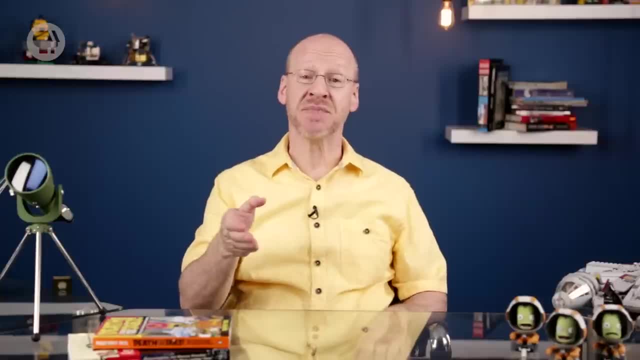 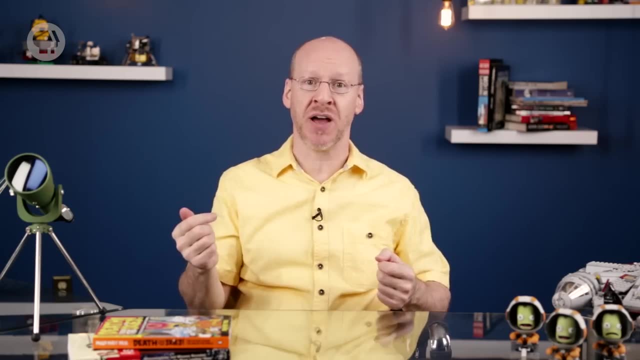 a few very narrow rings. The gap is due to one of Saturn's moons, Mimas. If you're an ice particle in the Cassini division, you orbit Saturn twice for every one time Mimas goes around. This is called a resonance and it means that the particles at that location get tugged repeatedly. 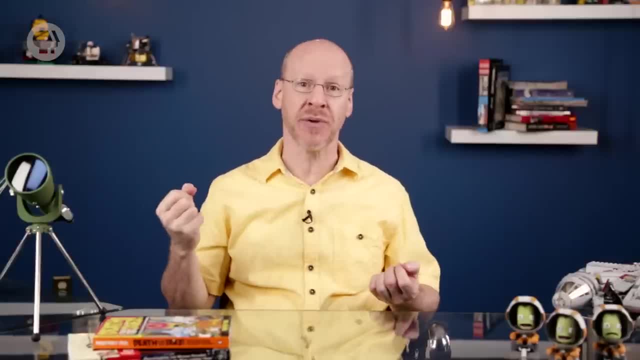 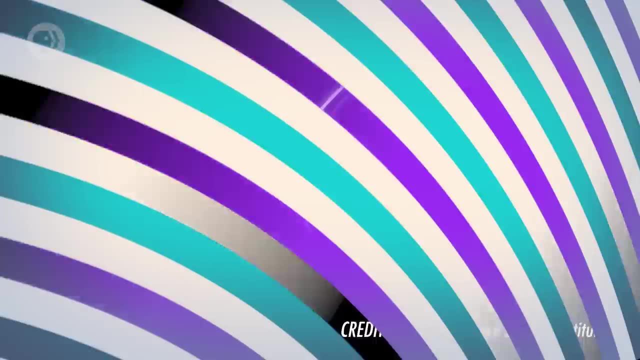 by the gravity of Mimas, which, in essence, yanks them out of their orbit. There are quite a few gaps in the rings, caused by moons. In fact, there are hundreds of ringlets in the main rings. Even weirder, the F ring is outside the A ring and is very narrow. just a few hundred kilometers across. It's kept that way by two moons, Prometheus and Pandora, orbiting just inside and outside the ring. They tug on the ring particles in such a way that keeps them confined to very strict orbits. If a particle wanders out, the moon's gravity drags it back in. 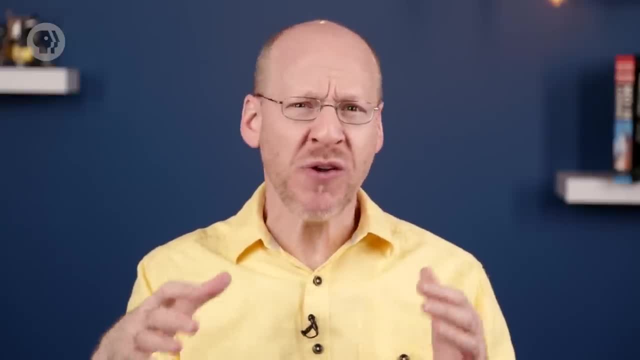 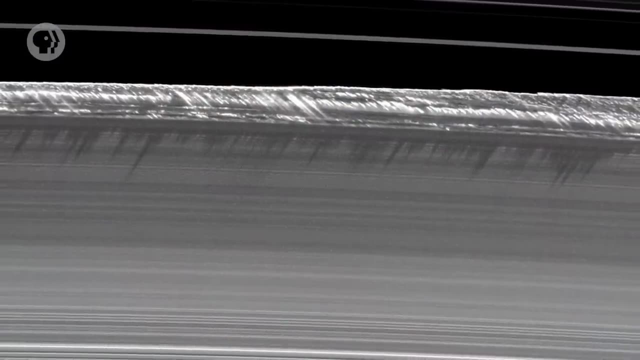 As the moons and ring particles interact, they can also create weird rippling waves in the rings And this is really cool. When small moons orbit Saturn on slightly inclined orbits, it can create waves in the rings, Tremendous vertical excursions that can reach. 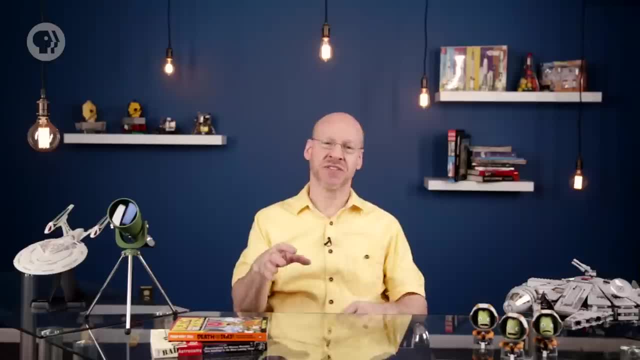 several kilometers per second, And this is really cool. When small moons orbit Saturn on slightly inclined orbits, it can create waves in the rings, Tremendous vertical excursions that can reach several kilometers per second. This is really cool. Saturn is weird, And so are its moons. I already mentioned Mimas, an icy moon that carves out. 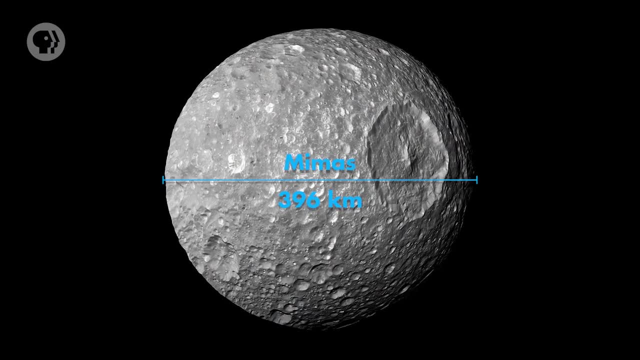 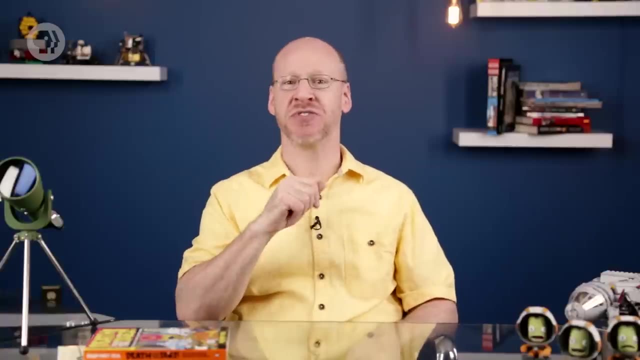 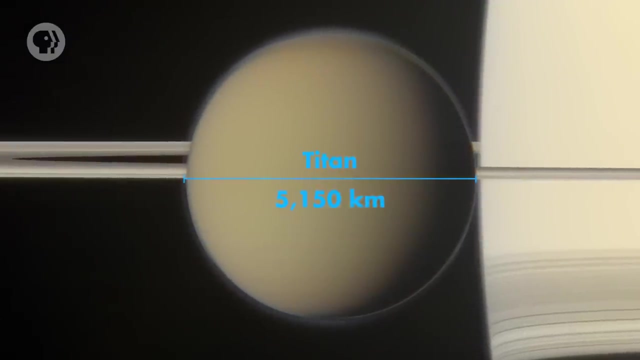 the Cassini Division. with its gravity It also suffered a massive impact long ago that created a single huge crater, making it look somehow familiar. But Saturn has two moons specifically you should know about. The first is Titan, a monster satellite that's actually bigger than Mercury, not that much smaller than Mars, And second, 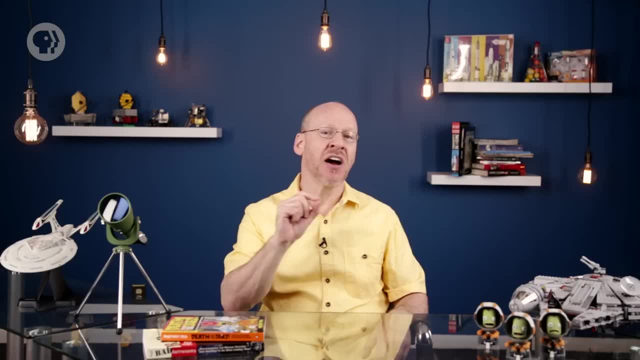 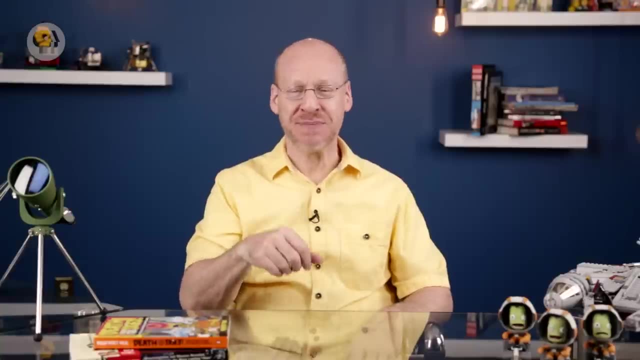 in moon size, ranking only to Jupiter's moon Ganymede. Titan not only has a substantial atmosphere- the only moon to have one- but it's thicker than our air on Earth. I wouldn't suggest breathing it, though It's mostly nitrogen with a smattering. 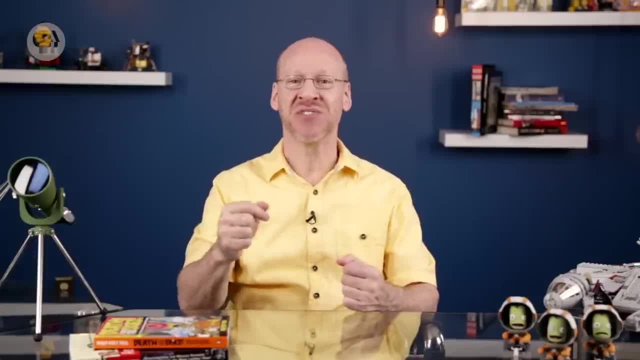 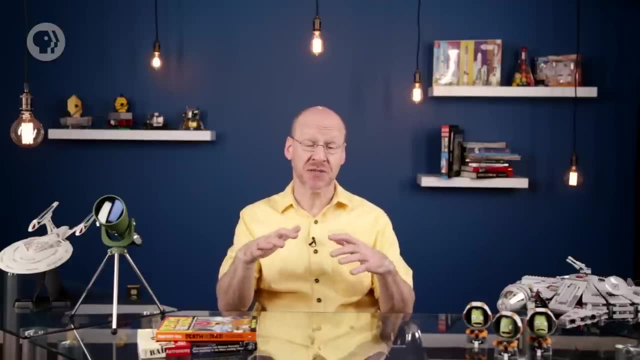 of methane and hydrogen. It's also 180 below zero Celsius there. Definitely don't stick your tongue on a flagpole on Titan. Titan's atmosphere has a thick layer of haze that prevents us from seeing the surface using visible light. But using infrared and radar though the Cassini spacecraft, which 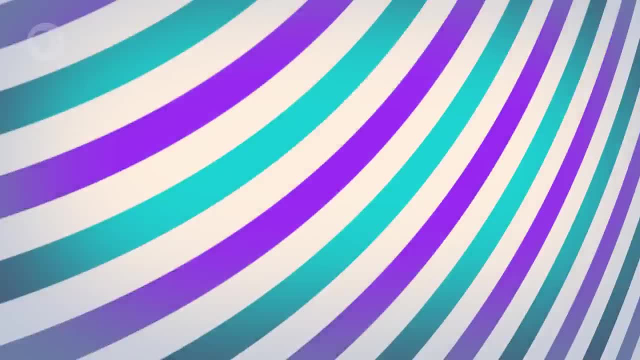 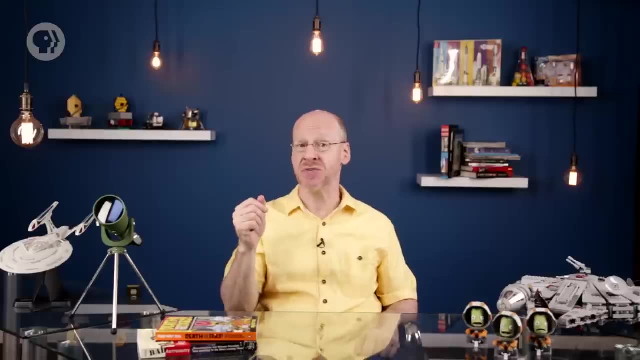 has been orbiting Saturn since 2004,. is able to map the surface. It also deployed a probe named Huygens to land on the surface of the Earth And on Titan's surface, the first time humanity had ever landed on an outer solar system- moon. 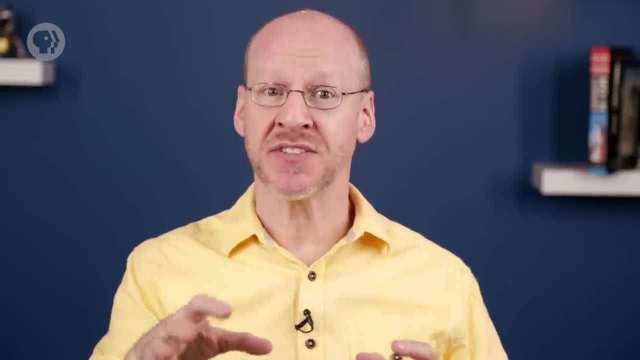 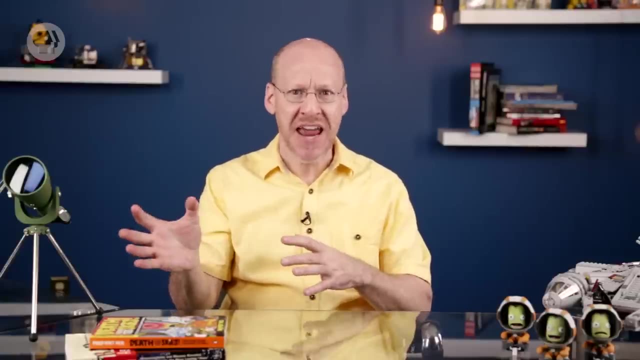 What they saw was an odd world: Earth-like in some ways and very alien in many others. Titan has wind-sculpted dunes, but they're made of hydrocarbon grains, not sand. There are hints of volcanoes that spew liquid water instead of lava. These are called cryovolcanoes. 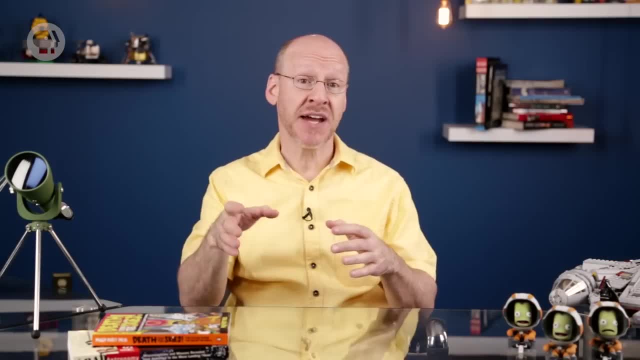 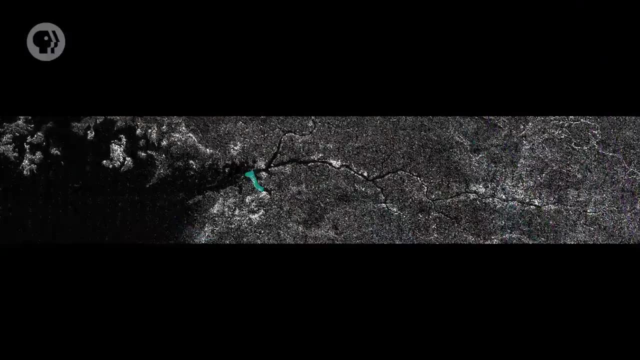 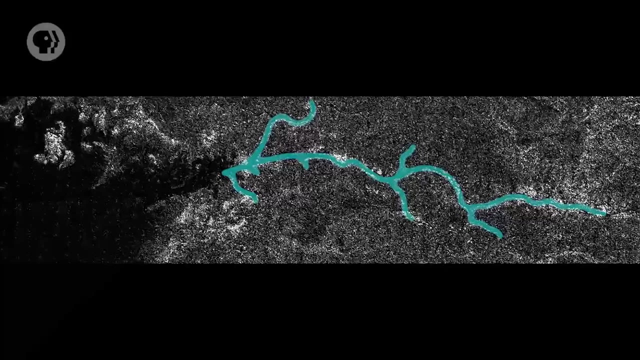 cold volcanoes, a term I love. This, together with measurements of Titan's gravitational field, have scientists thinking that Titan may have an underground ocean. Intriguingly, Titan also has long winding channels indicating flows of some kind of liquid on its surface, But it can't be water. it's far too cold on the surface for that. 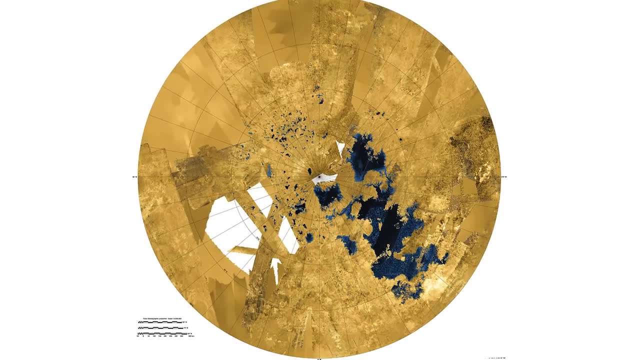 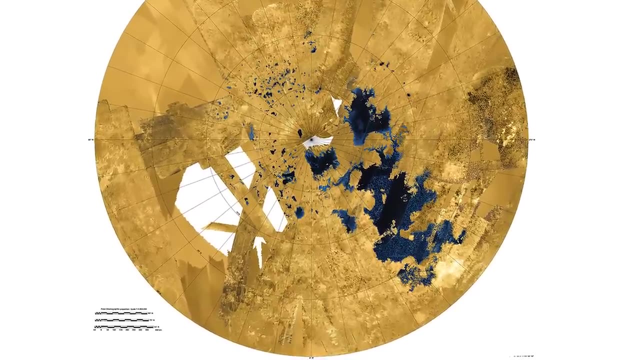 So what kind of liquid could it be? Well, Cassini also spotted quite a few flat regions near Titan's north and south poles. These have since been confirmed to be lakes of liquid methane, the first time any liquid has been seen on the surface of another world. 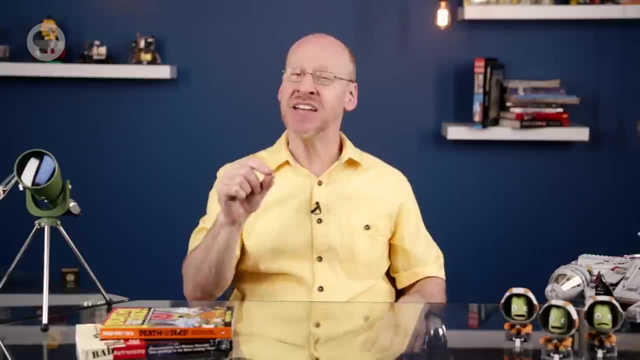 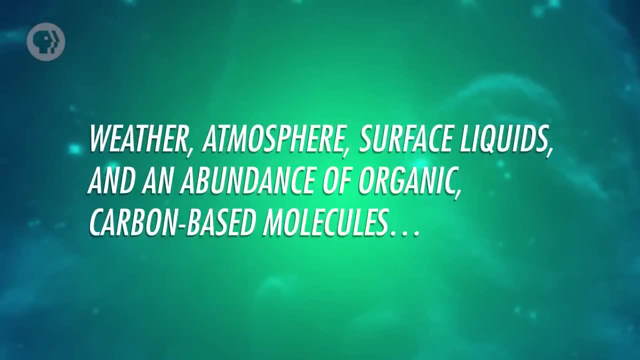 The shorelines of the lakes appear to change over time too, hinting very strongly that Titan has weather driven by methane as opposed to water here on Earth Weather, atmosphere, surface liquids and an abundance of organic carbon-based molecules. 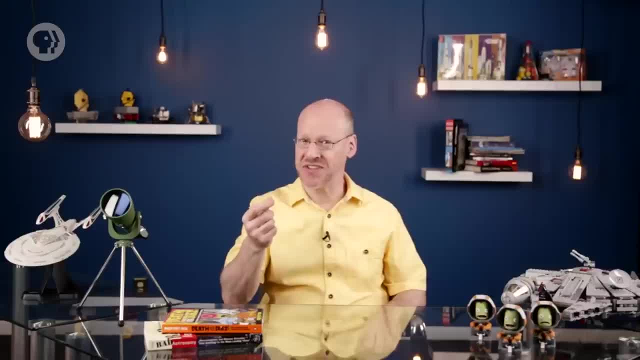 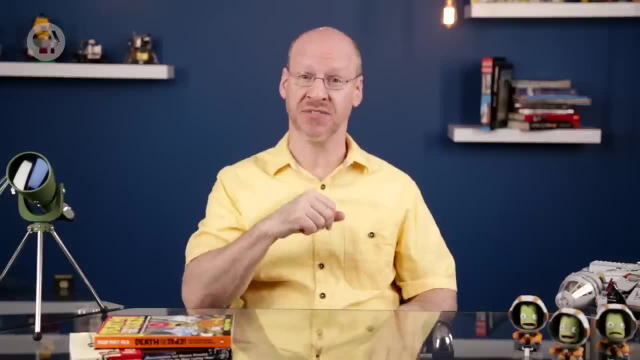 Could there be life on Titan? The conditions there are interesting. We obviously don't know yet, but it's an exciting possibility. And it's not the only Saturnian moon scientists are looking at for signs of life. Enceladus is a smaller. 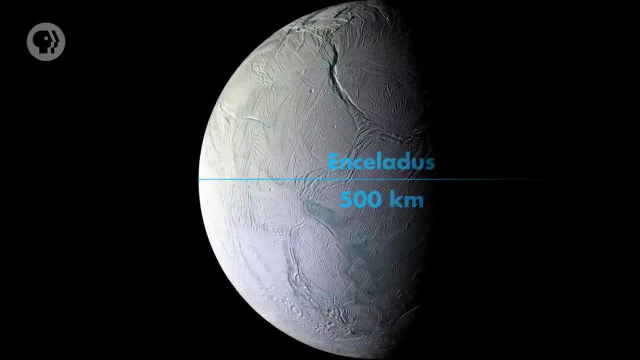 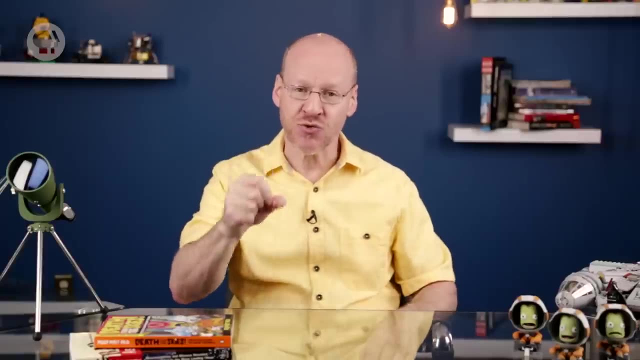 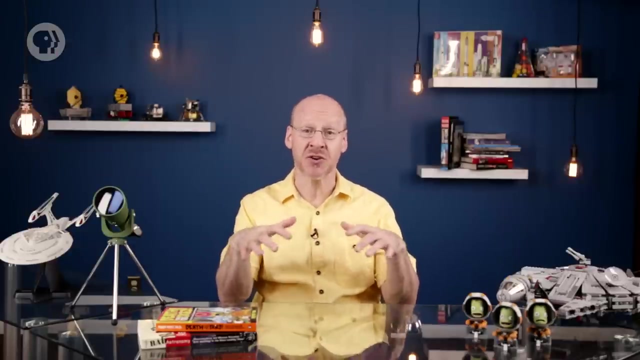 icy moon. about 500 kilometers across, about the size of my home state of Colorado or the southern part of England. It's collecting nearly all the light that hits it- a strong indicator. it's covered in water ice, Parts of it are cratered but other parts are very smooth, indicating some event resurfaced. 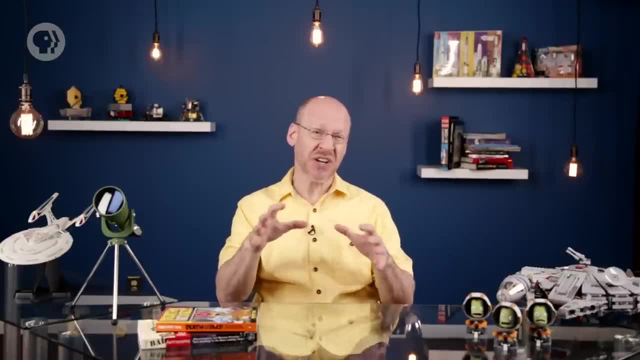 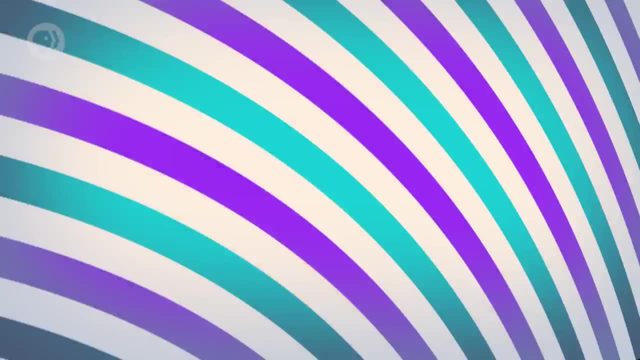 the moon. The surface also has an extensive series of cracks in it, much like Jupiter's moon Europa. Scientists suspected cryovolcanism and that was confirmed quite dramatically in 2005, when Cassini spotted active geysers of water spewing from the south pole of Enceladus. 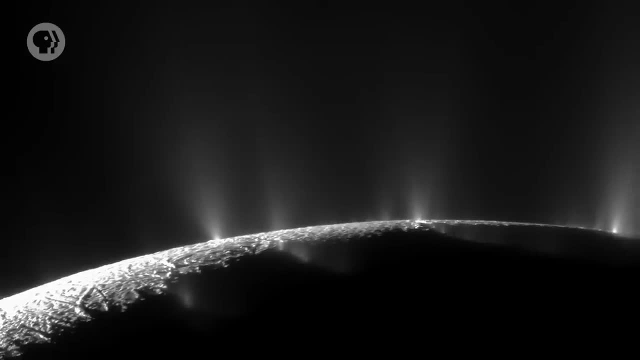 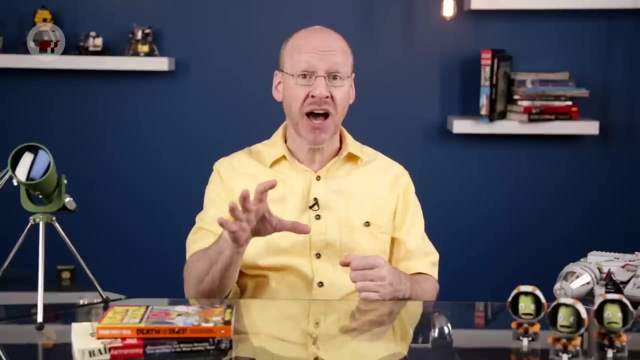 The water is erupting from a series of cracks, nicknamed tiger stripes, and is coming from deep under the surface. Like Europa, Enceladus has an undersurface ocean kept liquid by Saturn's ferocious tides, which squeeze the moon as it orbits the planet. The plumes reach several hundred. 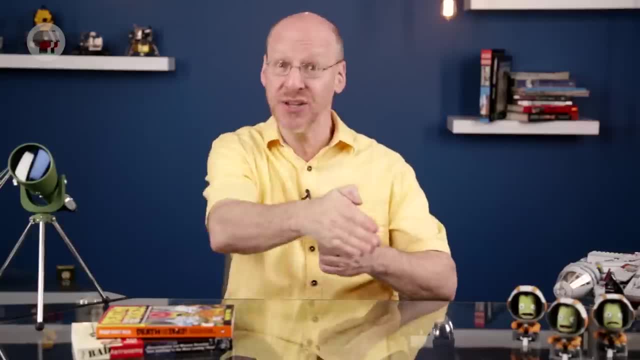 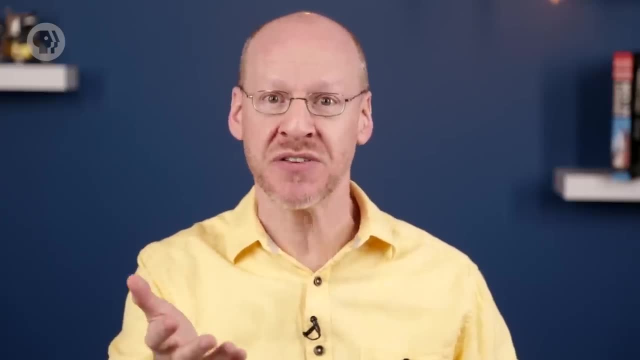 kilometers from the moon's surface, and Cassini even flew directly through the plumes and detected organic molecules. Could Enceladus be yet another harbor for life in the solar system? Again, no one knows, but I'd put it in the top three places to look, including Europa. 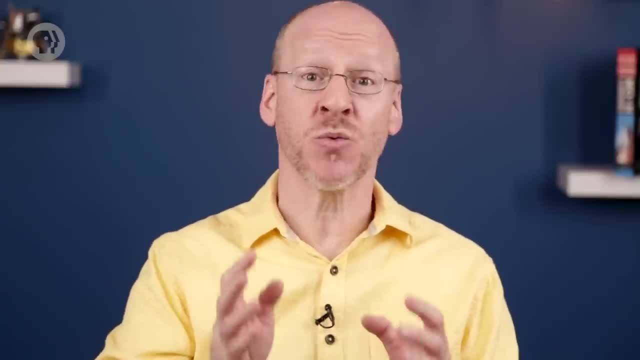 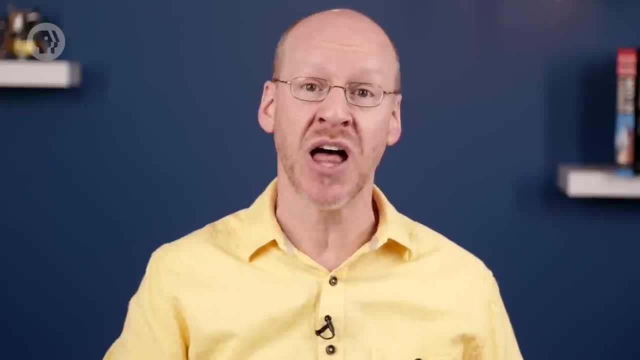 and Titan. It's weird, isn't it? We've always looked for planets, but we don't know where they're located. We've looked for planets where conditions were like conditions here on Earth, but it turns out extremely cold. moons may be the best places to seek out new life. Saturn has a huge retinue of other moons too, and they're all pretty weird. Iapetus is shaped like a walnut, with a tall ridge of mountains encircling its equator. No one's quite sure how that formed. Hyperion looks like a huge piece of styrofoam that's been hit repeatedly with a BB gun. 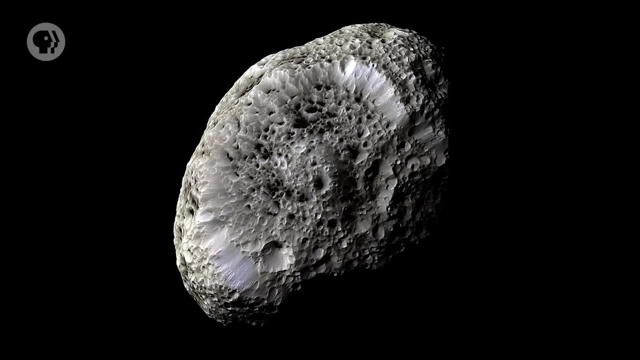 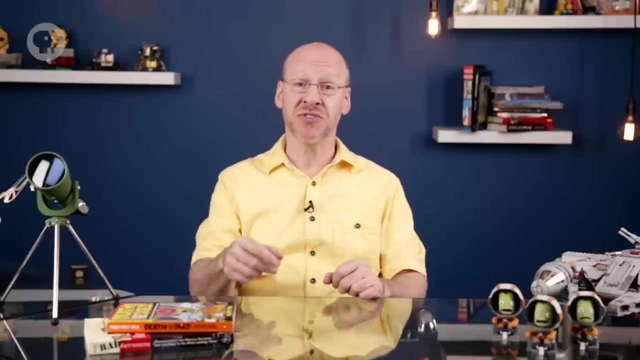 And that's not a bad analogy. since it has such a low density, it's likely to be extremely porous, like a sponge. A lot of Saturn's moons orbit the planet backwards retrograde, similar to several moons of Jupiter. These may be captured asteroids or even Kuiper belt objects- giant chunks. 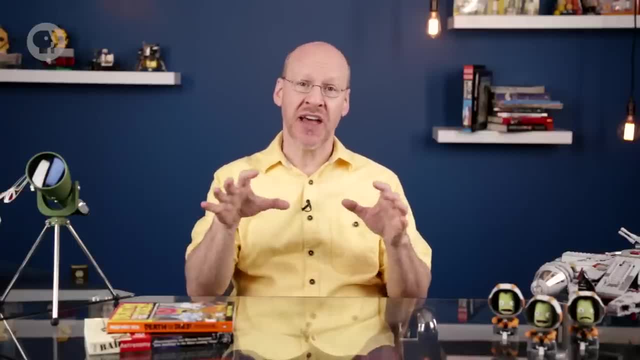 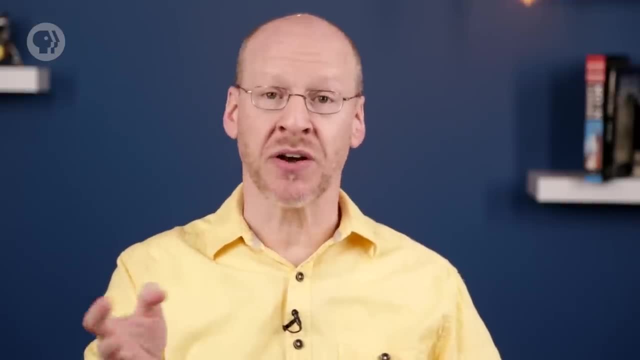 of ice. that we'll learn about very soon in a future episode. All in all, Saturn has over 60 moons we've discovered so far. I want to add a personal note. When you ask astronomers or astronauts what got them started, what was the very first thing that happened to them to inspire them to do what they do?